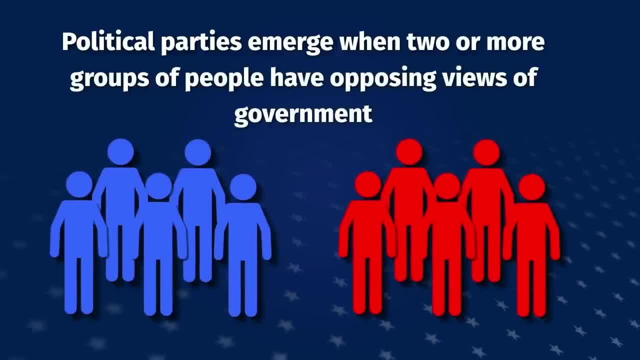 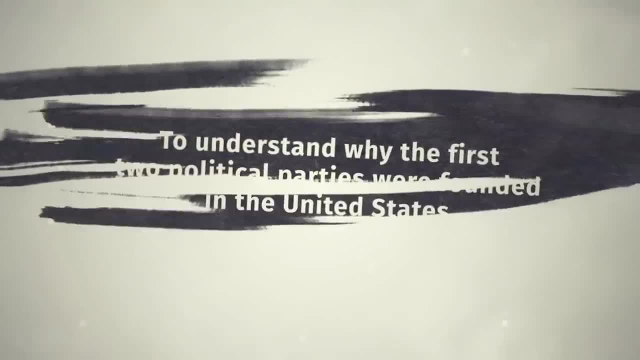 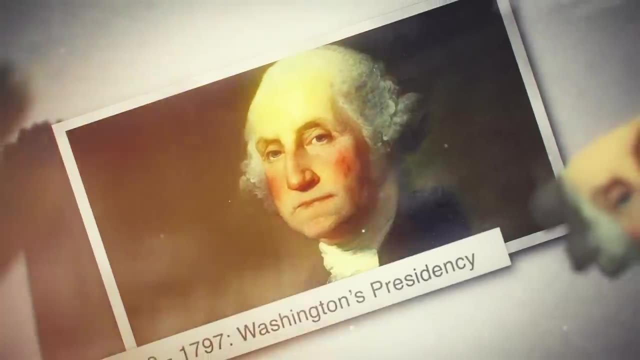 In general, political parties emerge when two or more groups of people have opposing views of government and both want to gain power. To understand why the first two political parties were founded in the United States, we need to go all the way back to Washington's presidency. 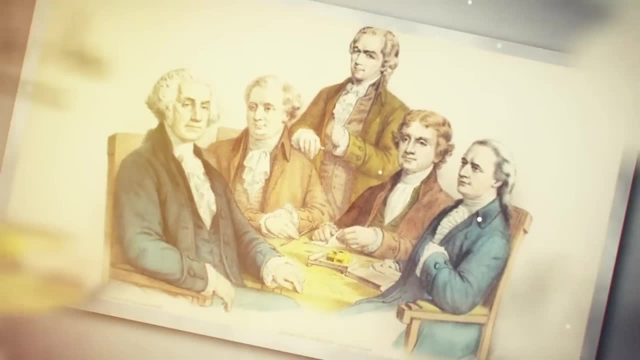 When he became president, Washington made sure to fill his cabinet with people who had a lot of power and a lot of power. And he made sure to fill his cabinet with people who had a lot of power and a lot of power. He also made sure to fill his cabinet with people who had different opinions, so he could make more informed decisions as president. 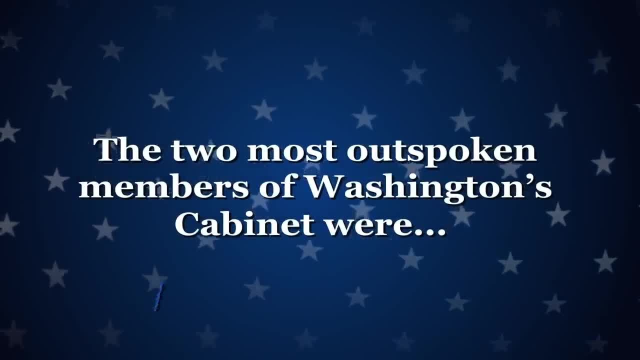 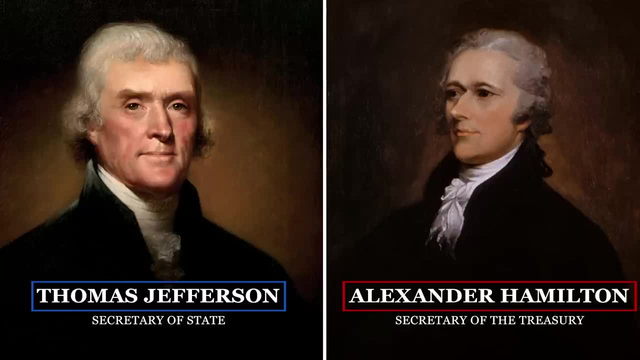 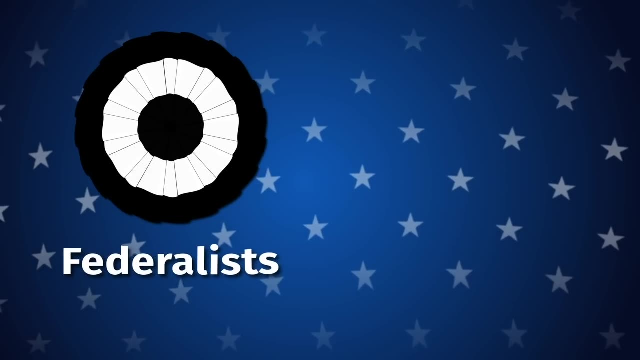 The two most outspoken members of Washington's cabinet were Thomas Jefferson, his Secretary of State, and Alexander Hamilton, his Secretary of the Treasury. Jefferson and Hamilton disagreed on almost everything, and their debates became the foundation for the first two political parties' ideologies. 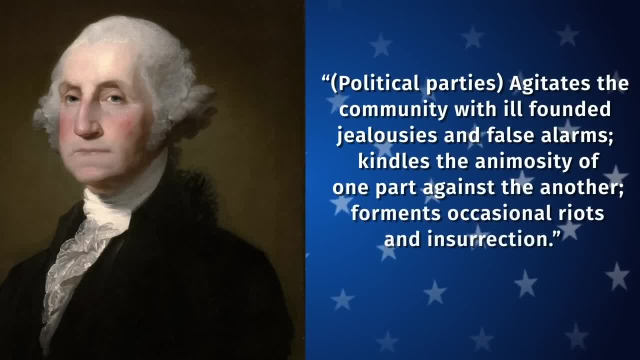 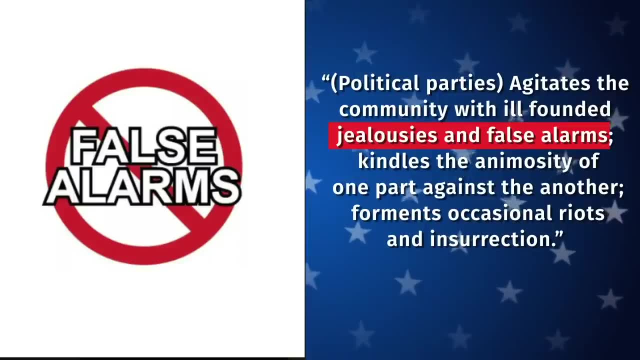 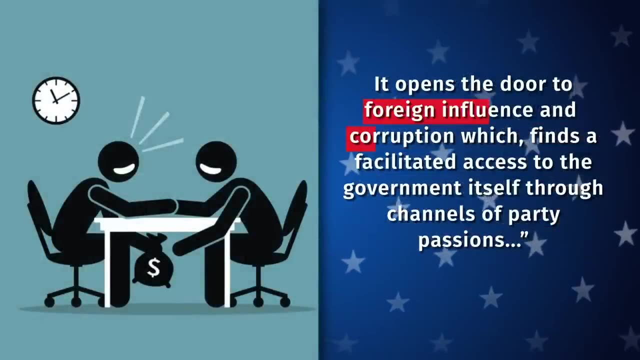 Washington warned that political parties agitate the community with ill-founded jealousies and false alarms kindles the animosity of one part against another ferments occasional riots and insurrection. It opens the door to foreign influence and corruption, which finds a facilitated access to the government itself through channels of party passions. In other words, Washington warned that political parties would lead to divisions and fighting among the people. This, he feared, could lead to foreign influence in the government and other forms of corruption. Despite Washington's warnings, the first two political parties emerged from the debates within his own cabinet and have since become prominent forces in American politics. 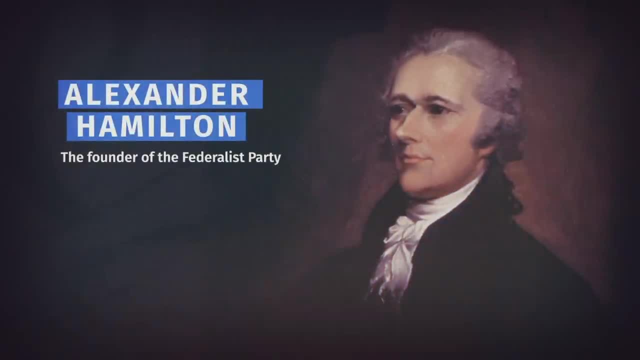 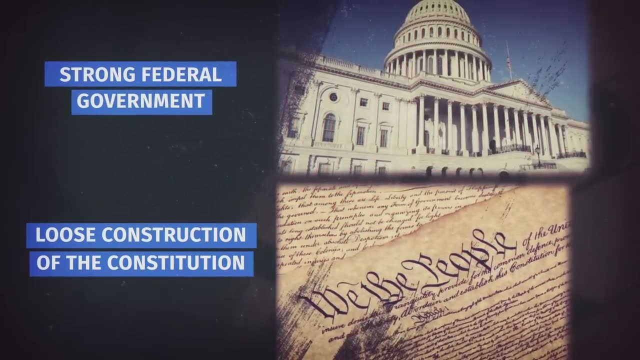 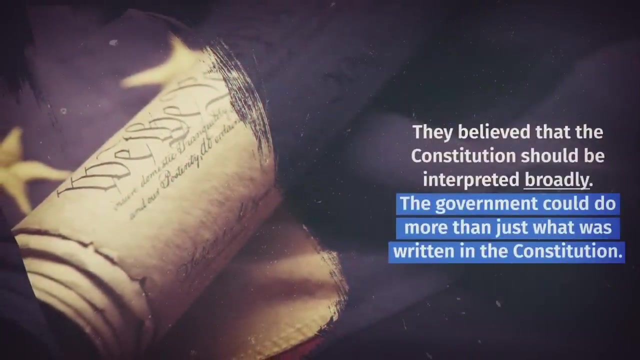 Alexander Hamilton is considered the founder of the Federalist Party, and John Adams emerged as another party leader. The Federalists favored a strong federal government and a loose construction of the Constitution. This means they believed the Constitution should be interpreted broadly. The government could do more than just what was written in the Constitution. 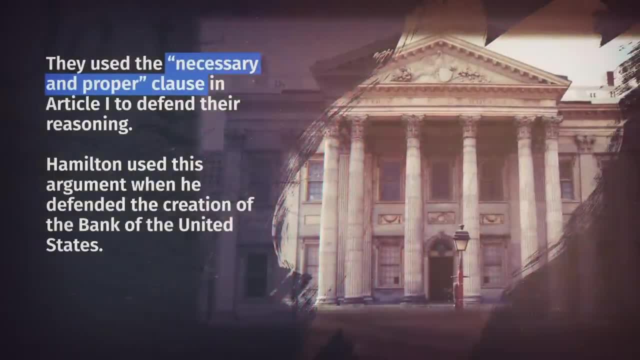 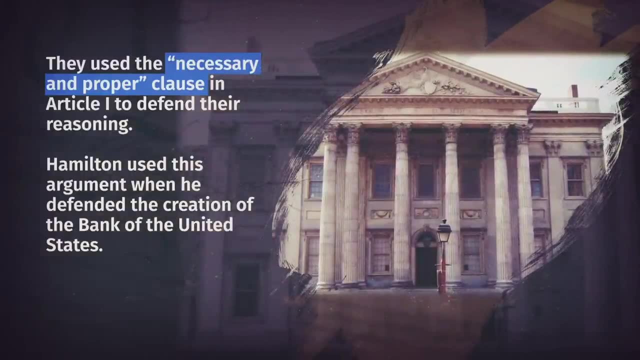 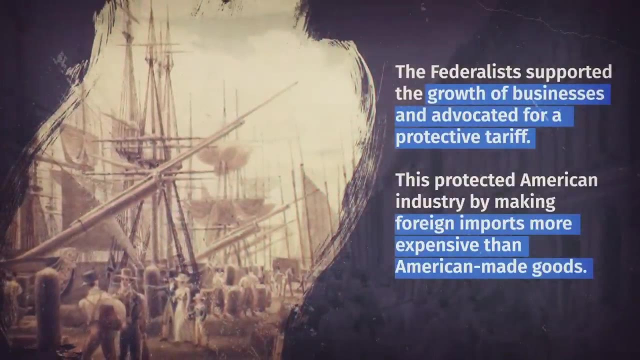 They used the Necessary and Proper Clause in Article I to defend their reasoning. Remember, Hamilton used this argument when he defended the creation of the Bank of the United States. The Federalists supported the growth of businesses and they advocated for a protective tariff. This protected American industry by making foreign imports more expensive than American-made goods. Finally, they supported alliances with Great Britain and their policies tended to support the wealthy. Federalists found most of their support in the northern states. Thomas Jefferson, Hamilton's enemy from Washington's cabinet, is considered the founder of the Democratic-Republican Party. 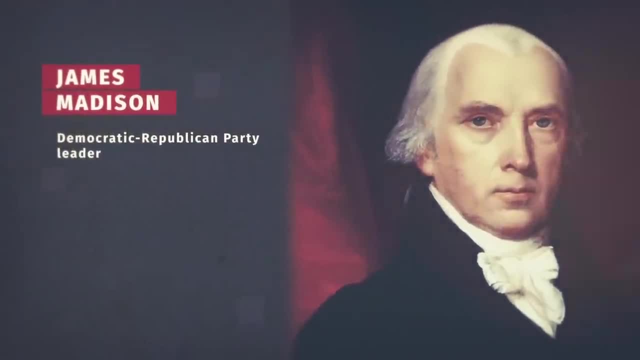 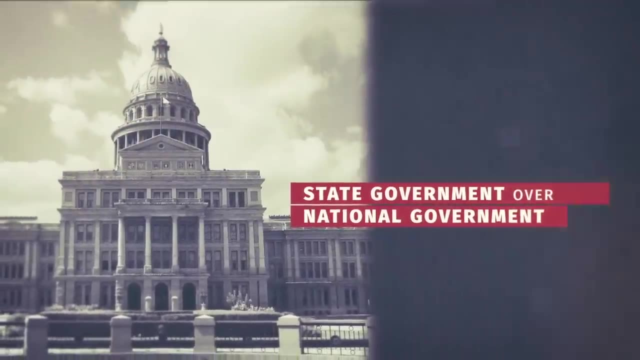 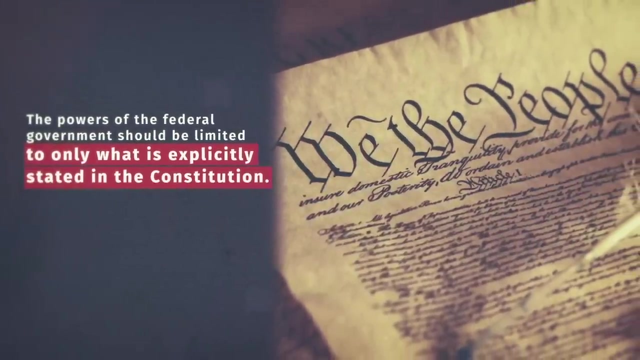 and James Madison became another early party leader. Unlike Federalists, the Democratic-Republicans favored strong state governments over a strong national government. They believed the powers of the federal government should be limited to only what was explicitly stated in the Constitution, which is known as a strict construction of the Constitution.